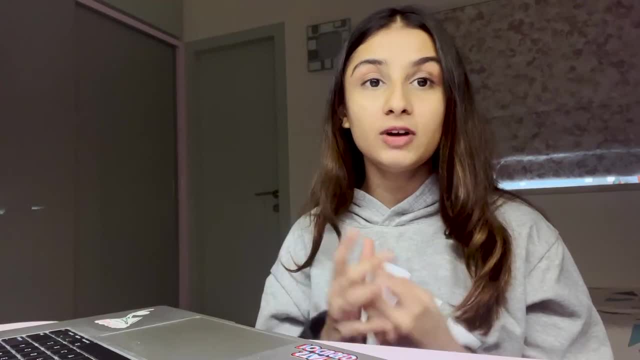 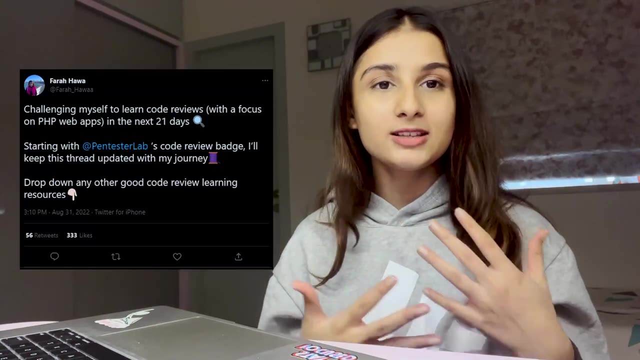 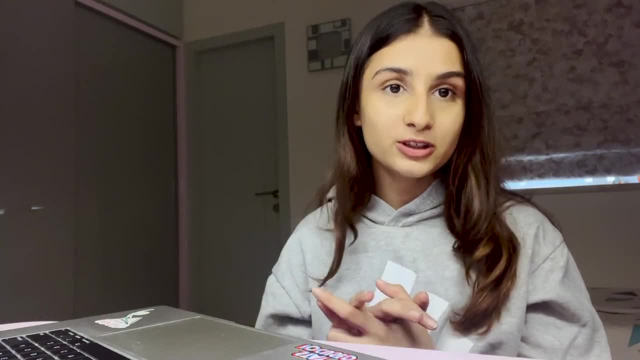 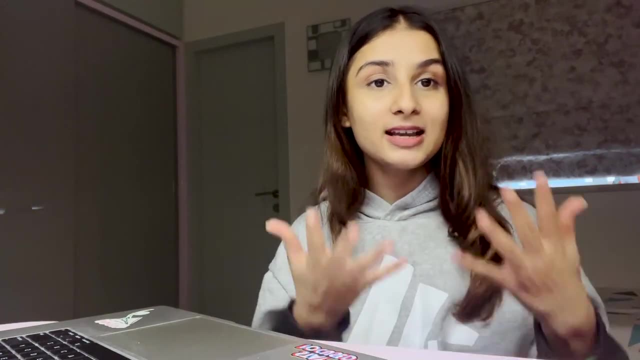 because I wanted to learn code reviews. This tweet got a really good response and I also updated the thread with my journey of learning. but I couldn't be very descriptive on Twitter, So I decided to also make a video sharing my journey. I linked the tweet below so you can. 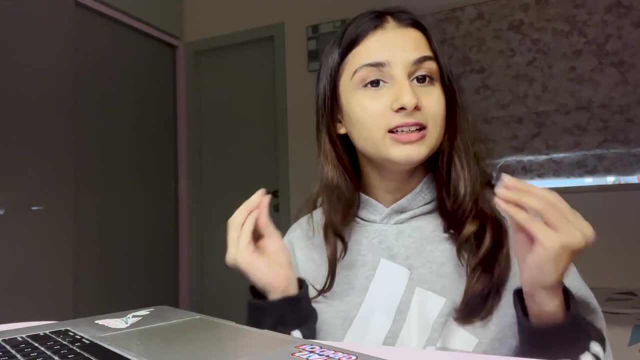 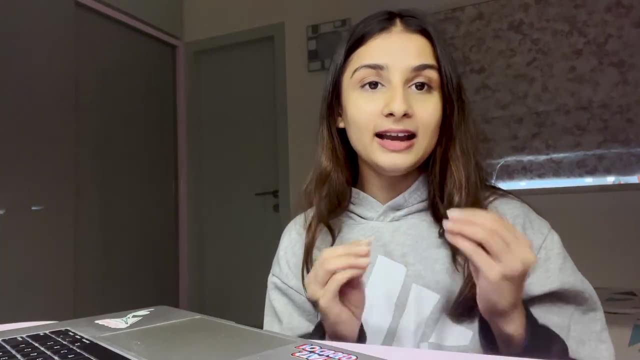 check it out, but this video is going to be a much more detailed version of that, And I'll also include some resources that I couldn't include in the tweet. So since I didn't know where to begin, I decided to look at Pentester coat lab, because that's kind of my go to resource. 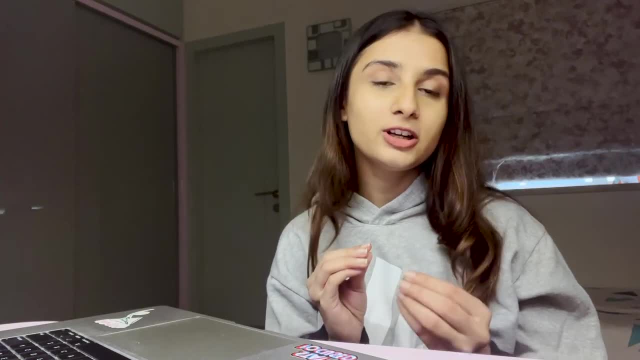 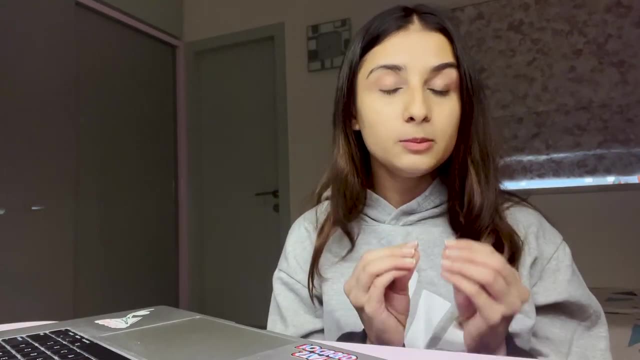 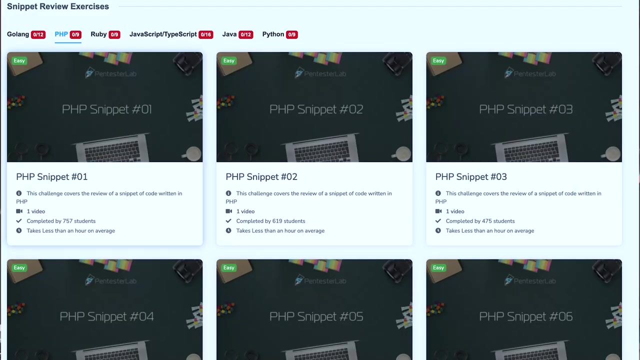 for web application, for anything web application related. so i decided to start with pentester lab. now, the resources for code reviews on pentester lab were a little bit limited. for example, i decided to choose php as my language to begin with, and they had only nine challenges for php. 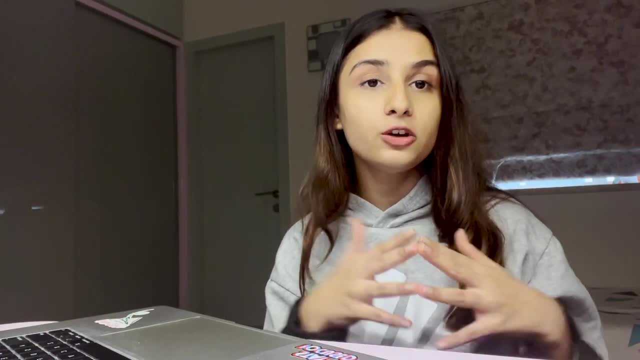 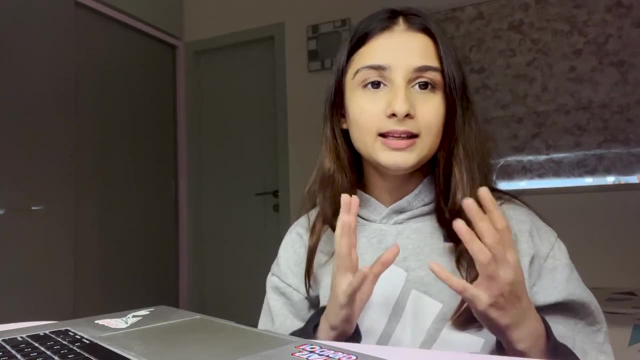 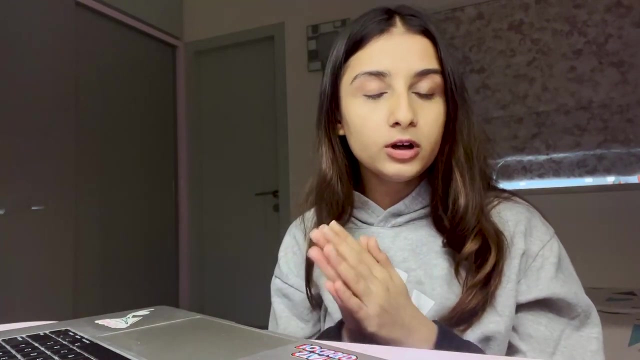 which i thought was a bit limited, but they had very good videos on how you can strategize and set your mindset before you learn how to review code, and i think that's very important, like i for me, because i didn't know what kind of mindset to go into when you look at a piece of code. so the 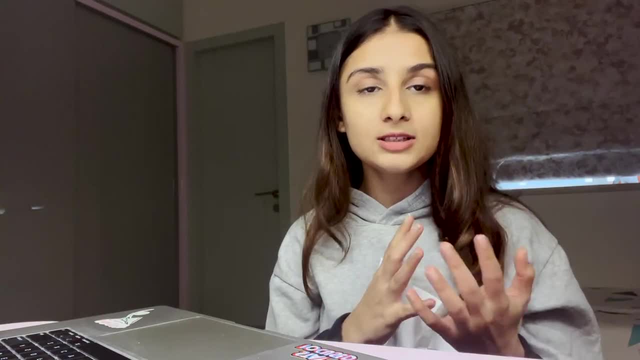 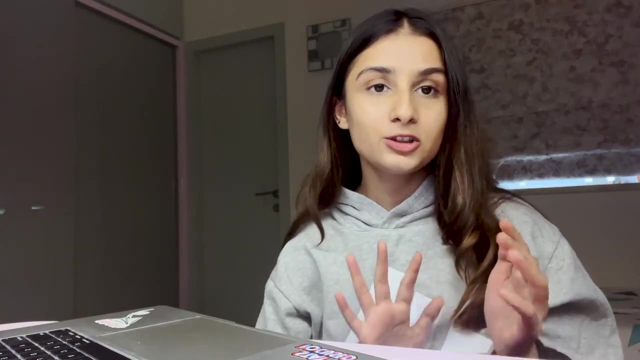 videos they had around strategy, around planning. they were a good start because it helped me build my mindset before i actually reviewed the code. the next resource that i decided to go with was suggested on the twitter thread, and that was sonar rules. now, since i was looking at php, i only looked. 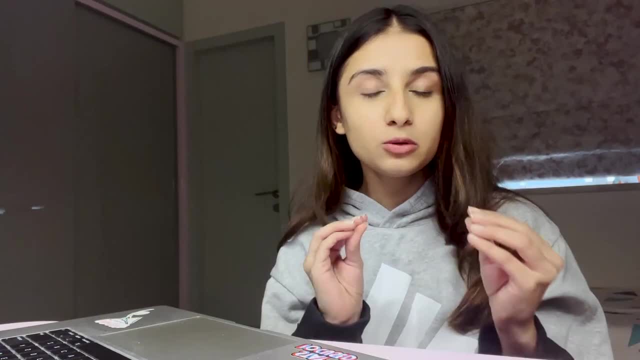 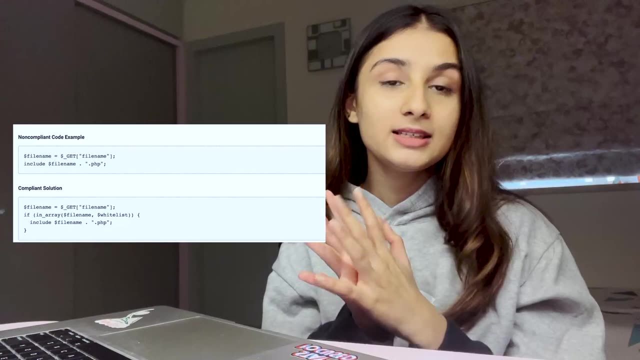 at the code review rules for php. now. code review rules are just like hacks, or they are like cheat sheets, uh, while you are code reviewing, so you will just learn about the basic areas of where flaws can come up. after going through this resource, i realized that the flow of input to output is the 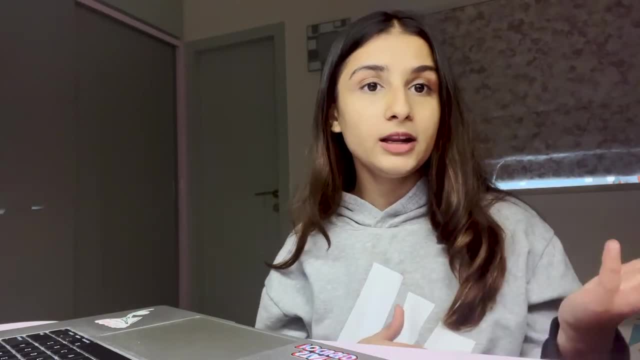 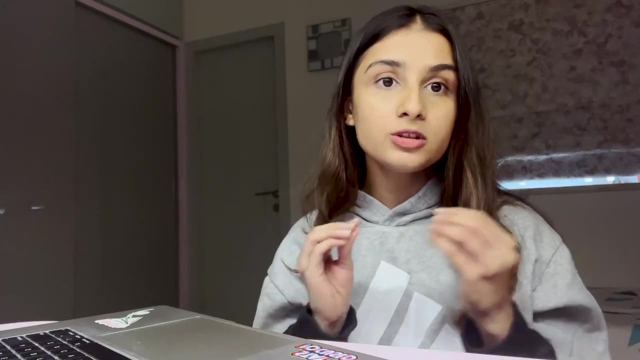 most important thing that needs to be reviewed, so to check where the user input is coming from- like cookies, headers, force data- and where the output is so kind of like source to sync. that's what you need to check when you're doing code reviews, and sonar rules will kind of give you like a checklist. 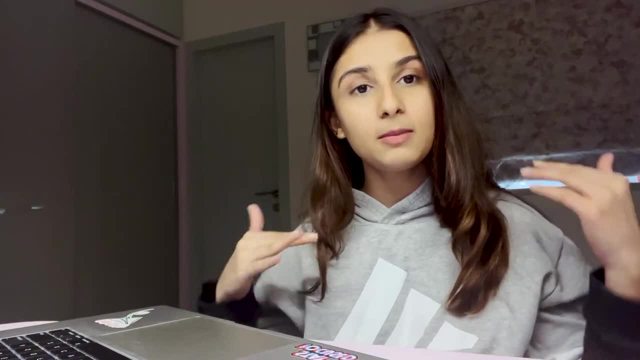 so when you go for code reviews, you have certain rules in the code review rules that you need to review. so when you go for code reviews, you have certain rules in the code review rules that you need to keep in mind, but keep in mind that these are basic and actual code will look a little bit. 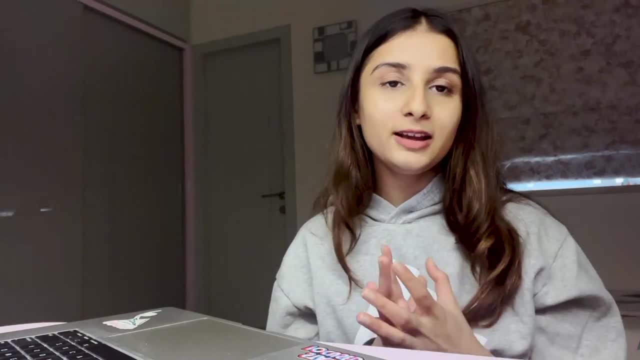 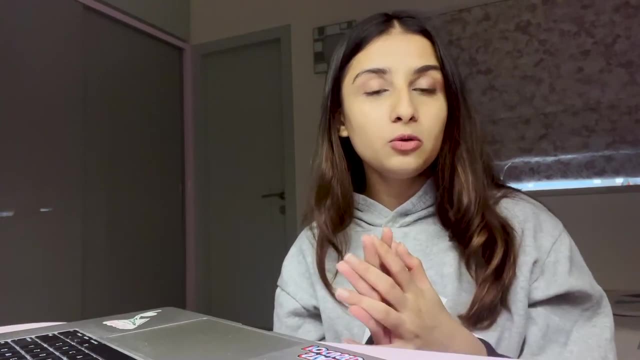 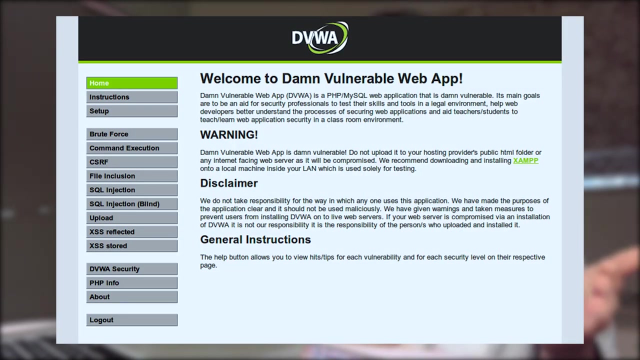 different and it won't be as straightforward. so the next thing i wanted to do was look at some actual code belonging to an actual application. so what i decided to do was look at code for vulnerable apps. like we have dvwa, where we generally look for vulnerabilities through. 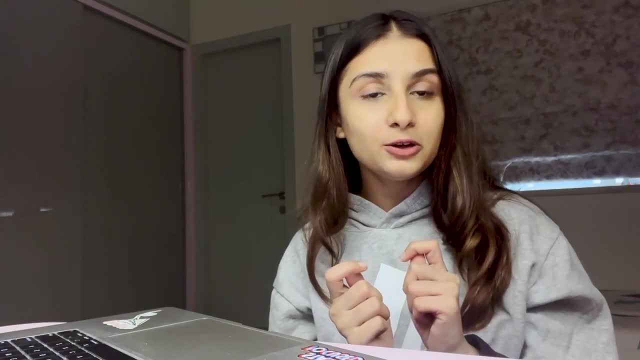 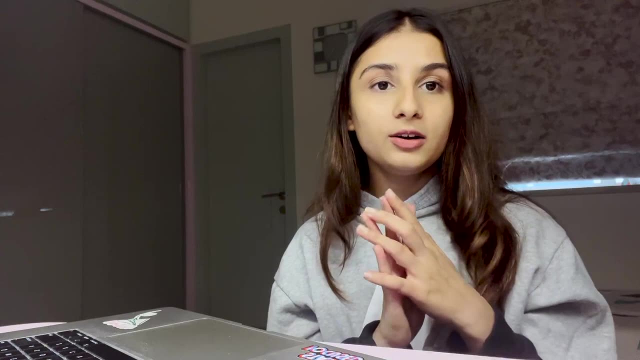 the web application itself. but what i decided to do was look at the code for the application. so i looked at the github repositories for these applications. i will link it below: uh, you can find the github repository for dvwa and then you can review the code. now, this was very useful for 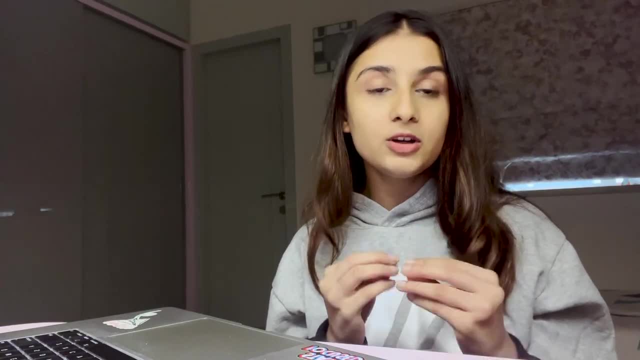 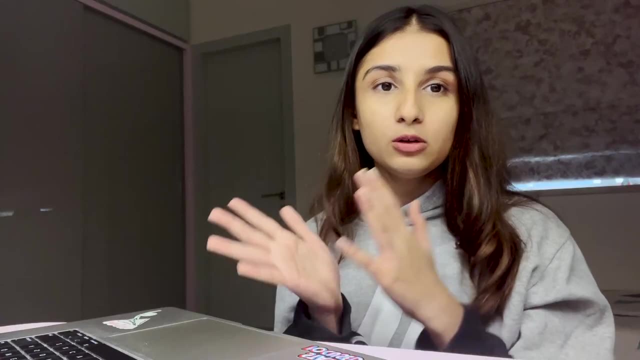 me and i think honestly, this was the best resource. uh, because it has different levels of vulnerabilities as well, like low, high, medium, so you can compare the fixes, for example, when you look at the low level. it will be a very straightforward piece of code which is easy to exploit. 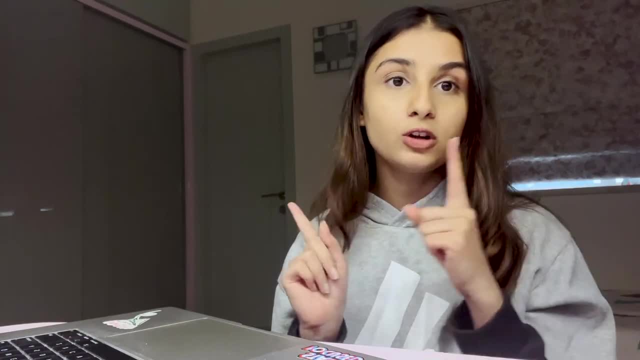 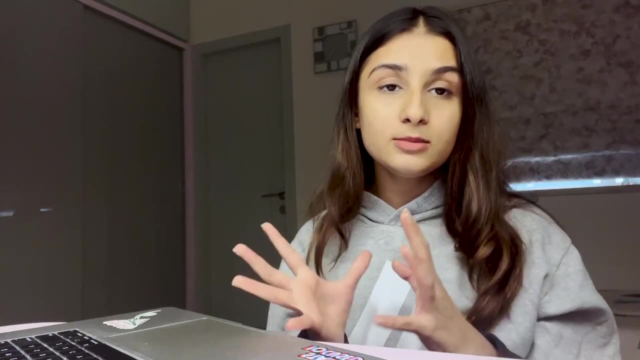 and then, when you look at medium, you'll realize what the fix was for the low level and how the developers were able to resolve it. this is a very important thing to know for code reviews, because at times there are security controls but the hacker finds a way to bypass it. 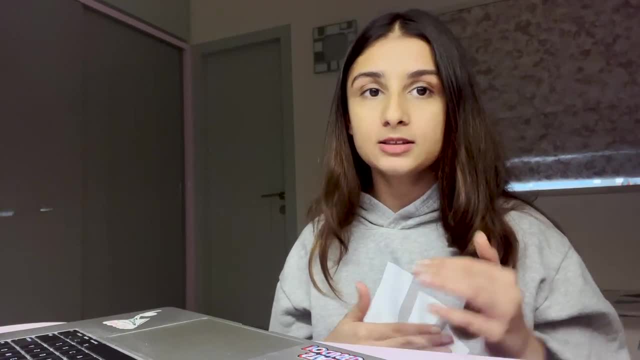 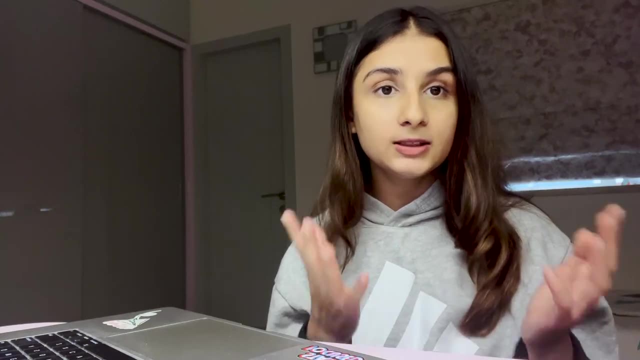 and dvwa was a good place to learn about these bypasses. so i chose php to learn code reviews, and dvwa was a good option, but you can also find applications for other languages, like for nodejs, or if you want to perform code reviews on oauth applications. i will also link a great github. 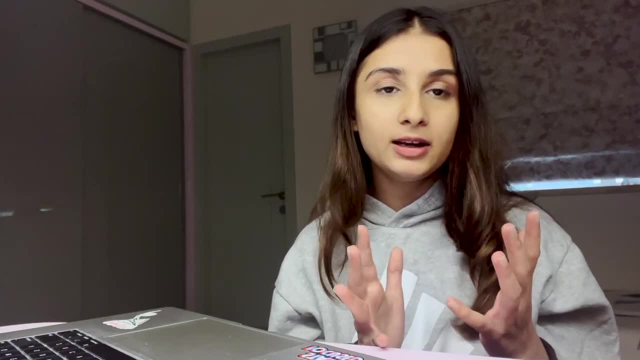 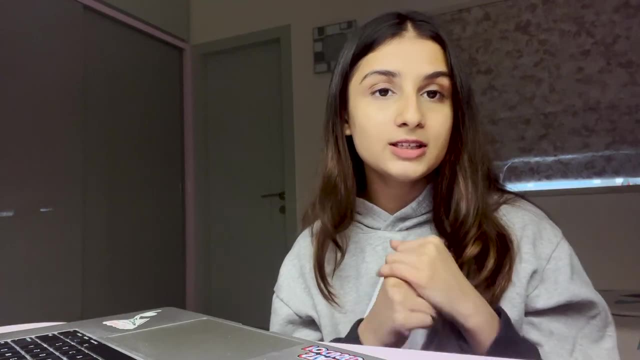 review on dvwa, where they also looked at the code for the oauth application that they had. you can also find vulnerable apis. for example, if you want to review a graphql application, you can find vulnerable graphql code repositories and learn graphql code reviews. i would also like to 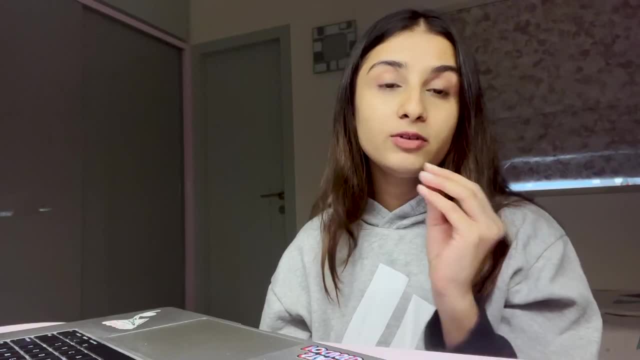 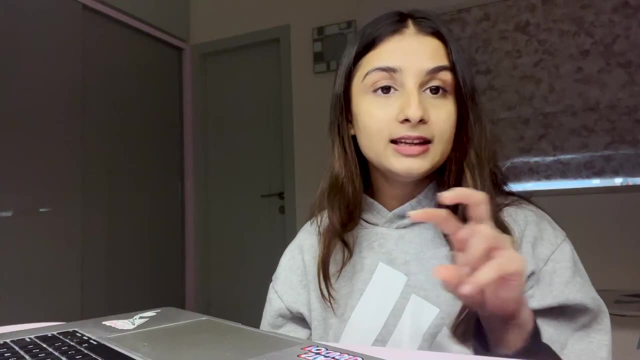 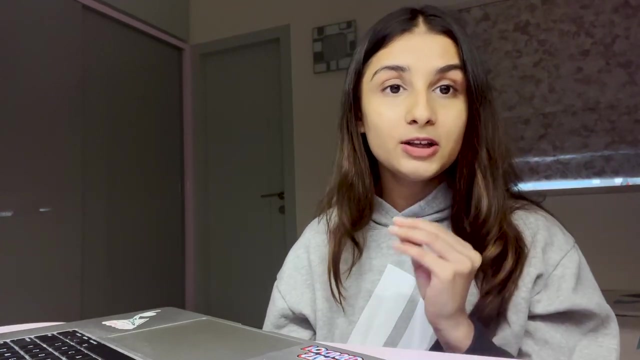 give a shout out to crypto cats playlist, i will link it below. they have made videos for every single bug on dvwa where they solve it through the web application and they also look at the code and analyze that for finding the root cause of the bug. you're using dvwa to learn code reviews. these videos are definitely worth watching after going. 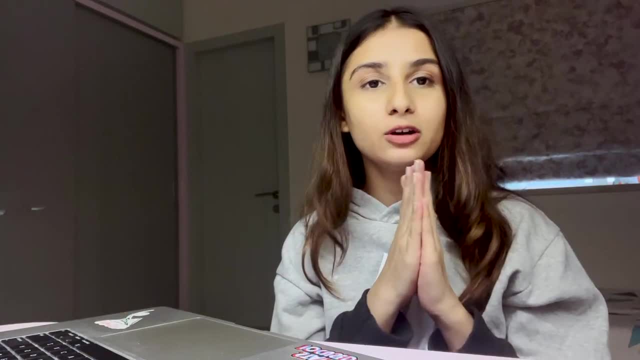 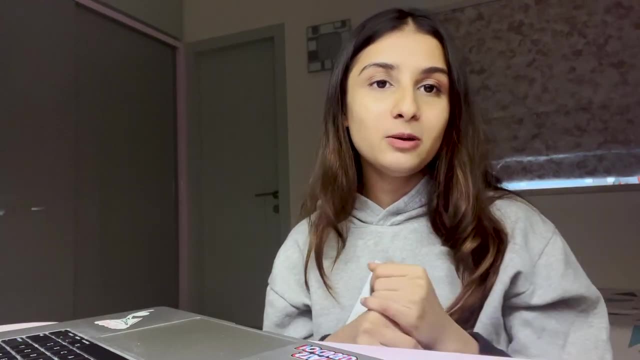 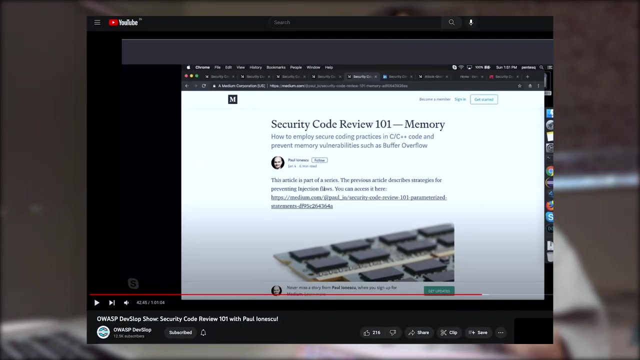 into this hands-on learning. i decided to go back and do a little bit more theory and watch a bit more videos about how people do their code reviews. so i want to tell you about this channel that i found at this point, called oas devslaw. they have some great videos about code reviews and different. 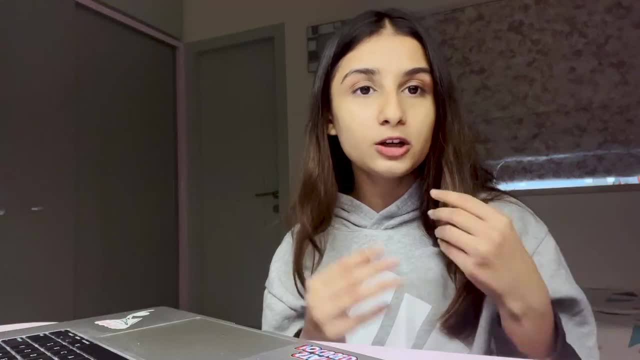 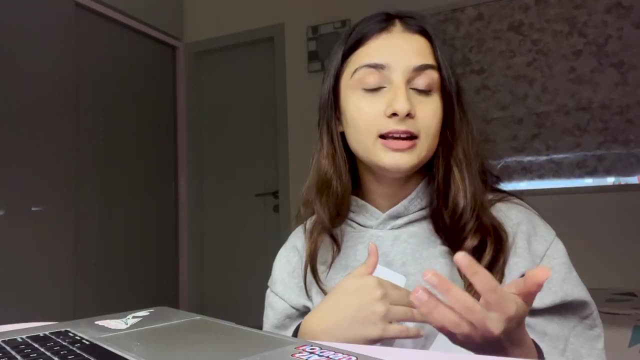 people who come onto their channel and walk the audience through their code review process. my favorite video was the one that was made by infosec au or shubham shah. he shows how you can analyze code reviews for offensive security, which is exactly what i wanted to do- another great video. 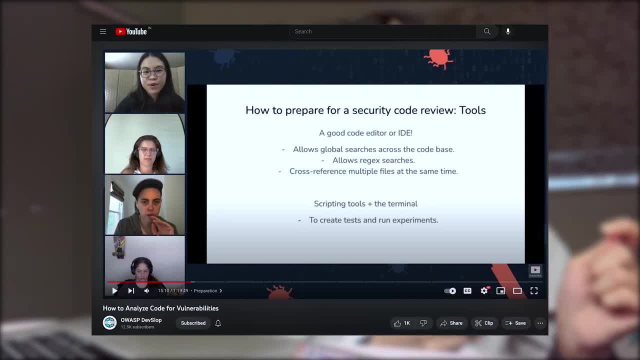 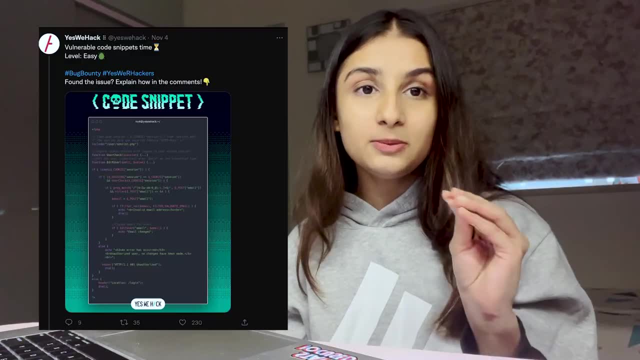 that they had was by vicky lee, where she also goes through her code review process. she also has a video about it on her own channel. i will be mentioning all the links in the description below. yes, we hack and integrity's twitter pages also started posting a bunch of code review challenges. 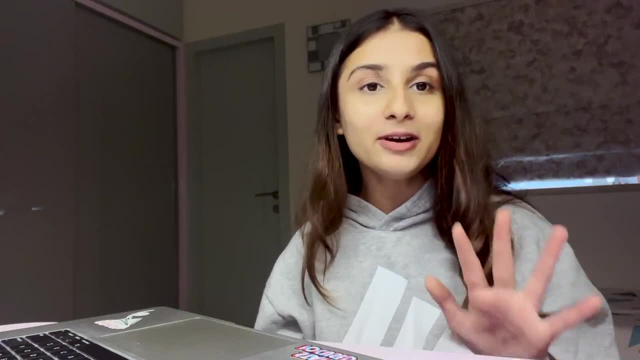 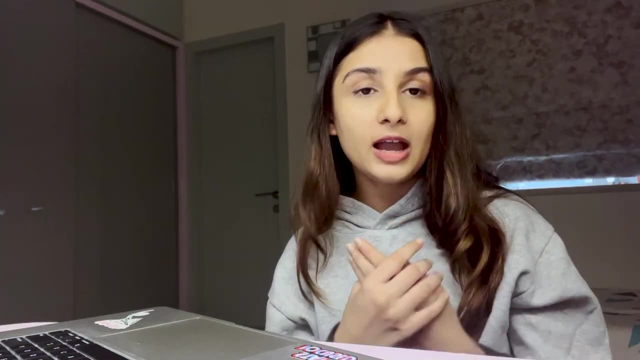 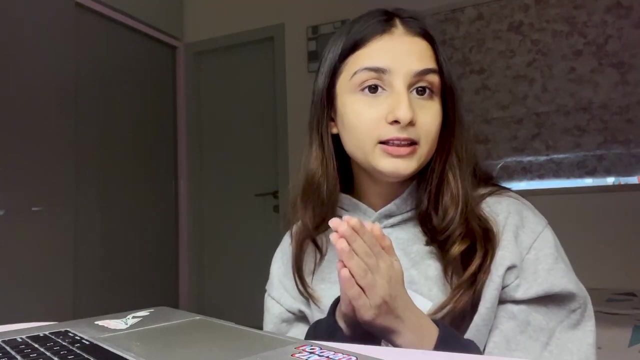 every week or a few days in a week, i'm not sure, but their challenges were a great way for me to just test myself and see how i was doing in my learning process. i was able to solve the challenges most of the times, especially the easy ones. i could see myself finding the root cause and finding the vulnerability correctly. so 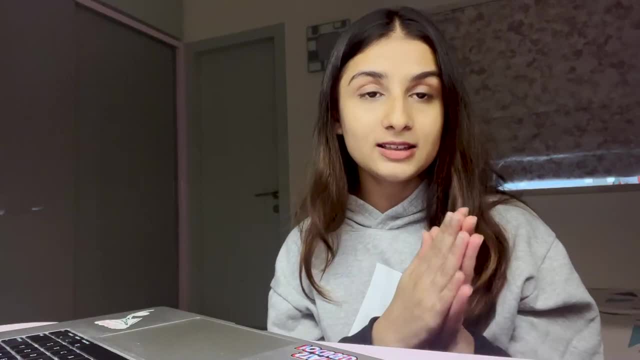 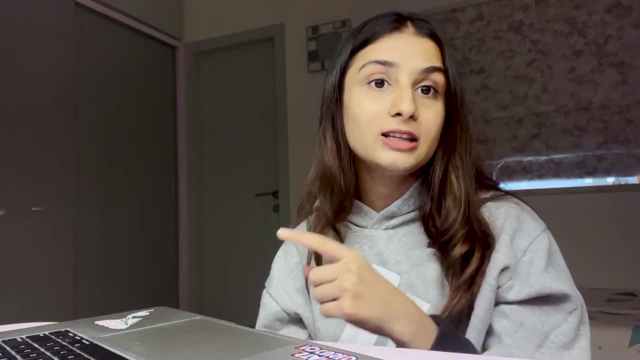 that was making me a little bit happy that i had made some progress in my learning journey. so if you want to look at those challenges, i would highly recommend that, while you're learning code reviews, also look at these challenges posted by integrity. and yes, we hack because this will. 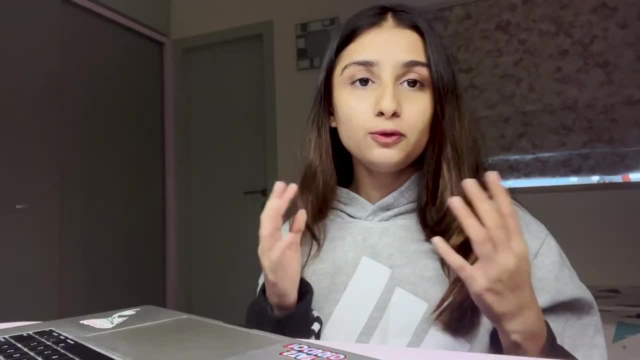 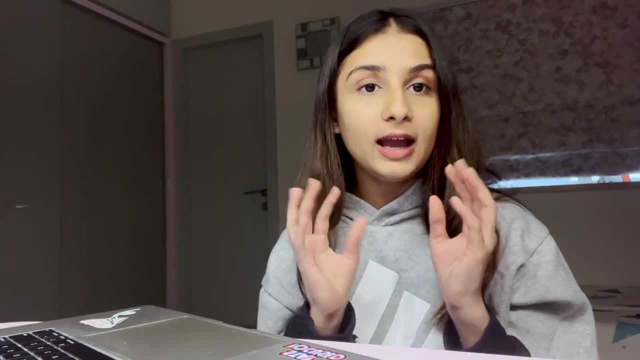 help you test yourself and see if you've learned anything. so from the oas devs love videos. i found the asset note blogs written by shubham shah about the bugs that he's found. so on asset notes blog page you will find write-ups of how he found bugs for bug bounty programs through code reviews and 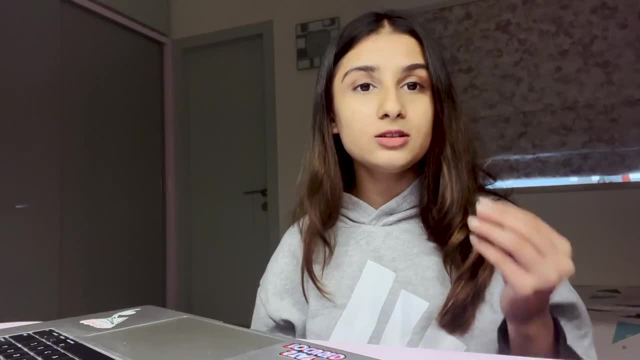 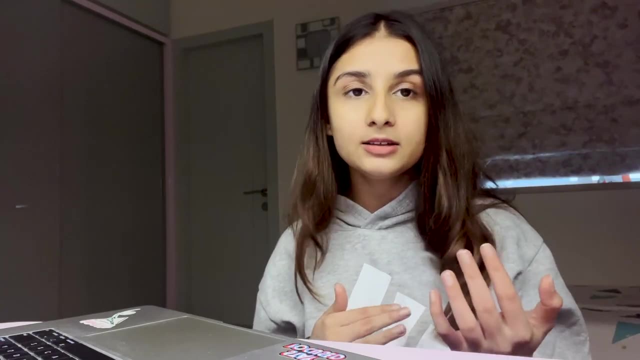 how he was able to obtain the code. so these write-ups were a good way to see how people were finding bugs in actual targets that would bug bounty targets. so they were a little bit more hardened than the vulnerable apps that we were practicing on the web. so i hope you guys found it. 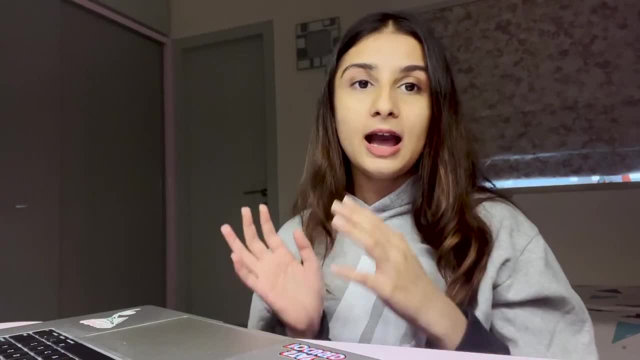 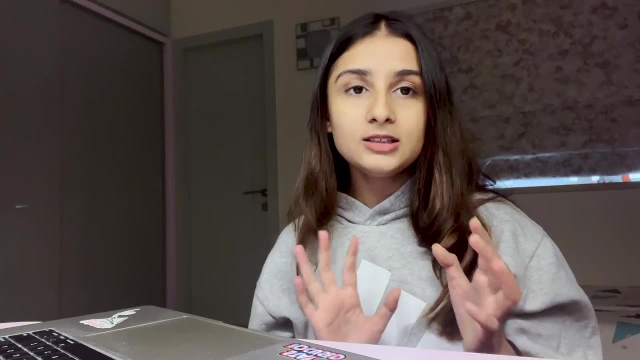 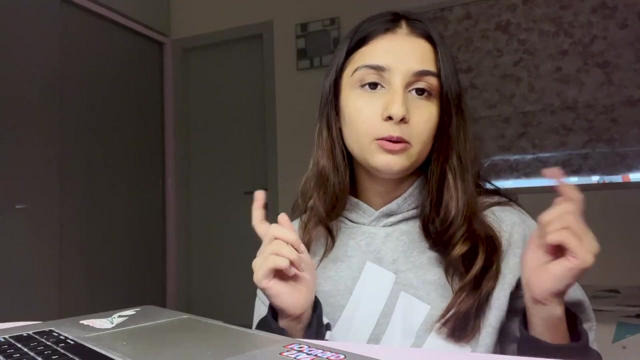 helpful and i will see you in the next video. bye, bye on earlier. so i would highly recommend that at an advanced stage, after you've done the basic code review work, that you go to his blogs and check them out. so the last resource that i want to talk about is the oas code review guide. it is a book. it is for free. you can find it online. i will 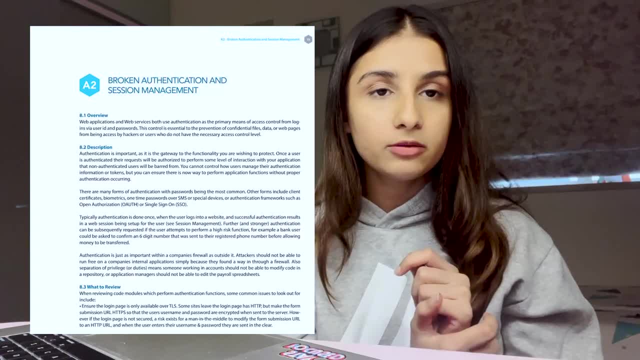 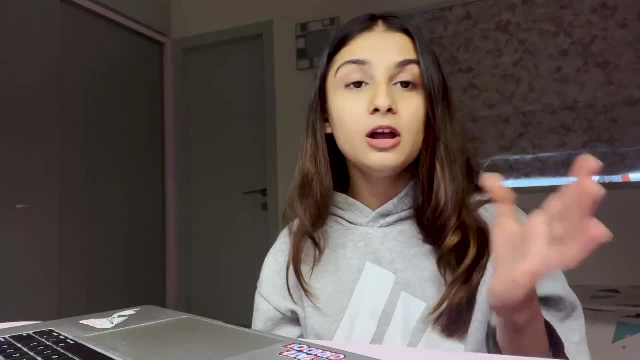 also link it below. this book has a lot of theory about code reviews and it goes through each oas category and how you can do code reviews for those categories, for example, broken authentication and session management. and how you can do code reviews for those categories, for example. 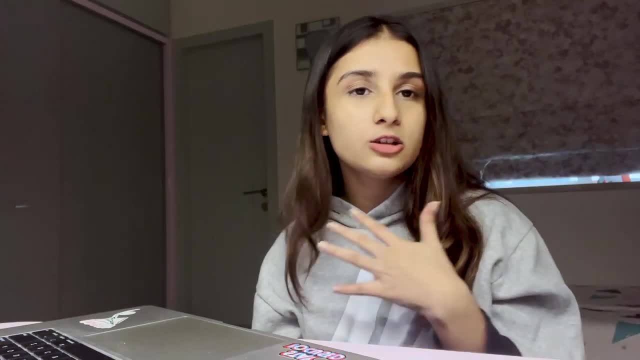 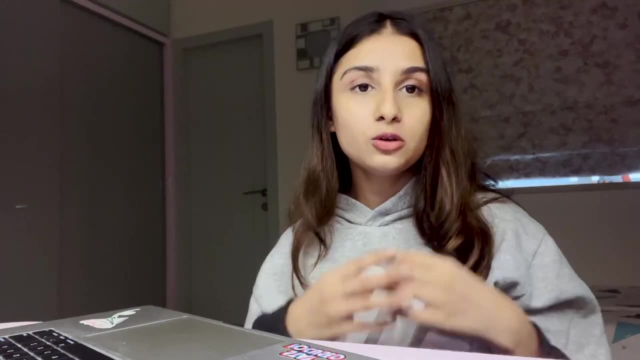 how you can perform code reviews for those bugs or broken access control information disclosures. so this was also a good way to kind of set my mindset before i go into code reviews. so what i do to keep myself updated after going through all these resources to keep myself updated with code. 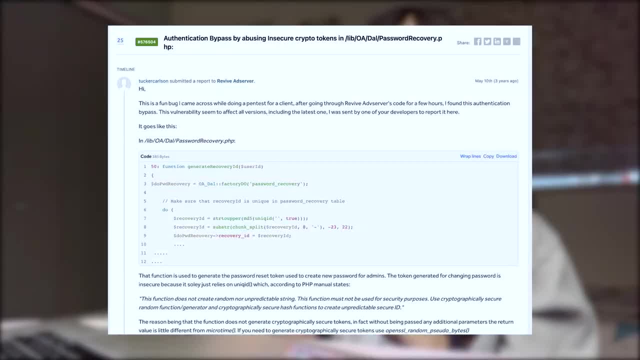 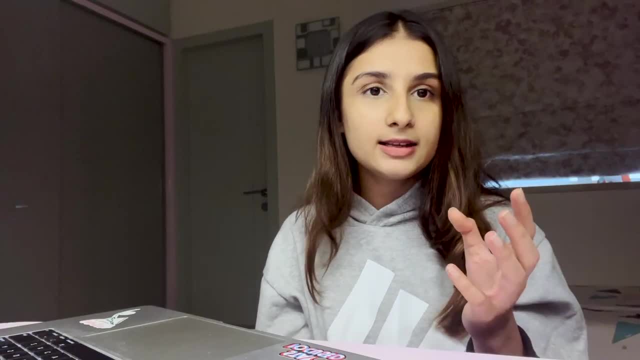 reviews and how bugs are fixed. so hacker one has hacktivity, where they disclose reports that have been fixed, and some of their targets also have github repositories for analyzing code. uh, i have to admit that i don't know if you guys are familiar with github repositories, because i have a lot of 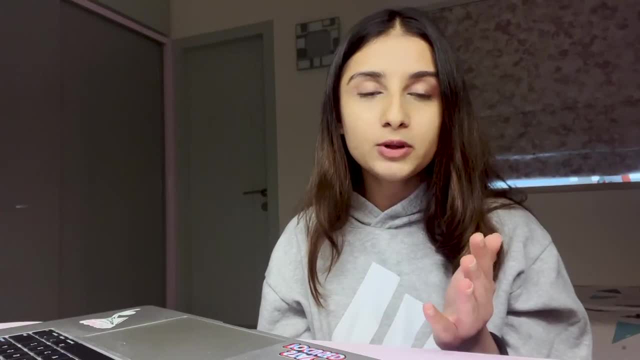 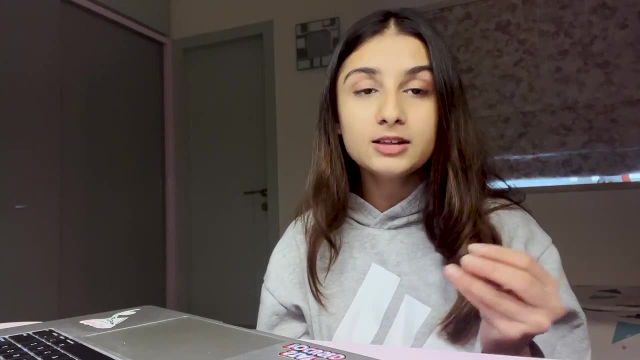 experience with github, but very few bugs that are disclosed are actually for code reviews, but you'll find one or two occasionally, so i would suggest you look at those reports to see how bug hunters were able to find bugs doing code reviews and another good way to keep learning about code. 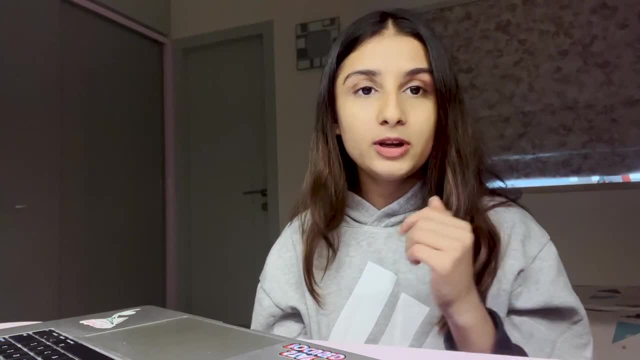 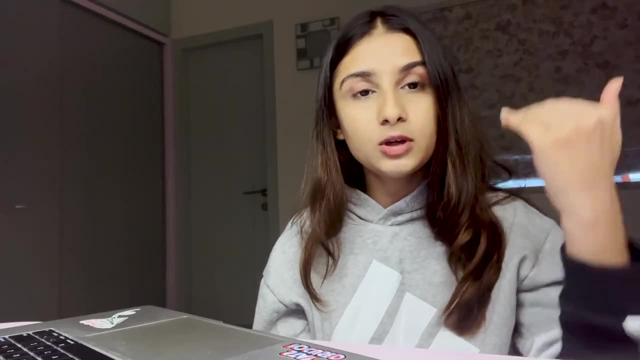 reviews is seeing how cves are fixed. so when you check online, if you go to exploit tv or anywhere where you can see how a cve was fixed in the code, uh, if you can go to their github repository and also see the public changes that they've made, you'll see how they've fixed the code. 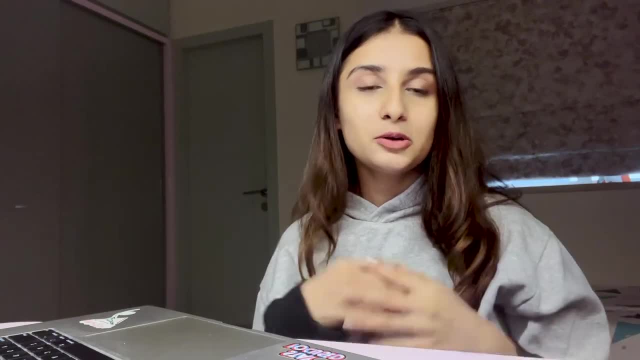 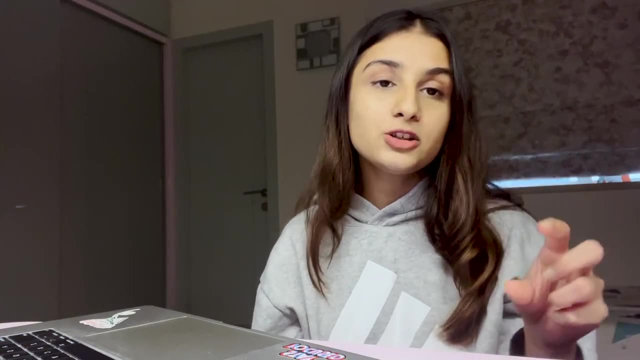 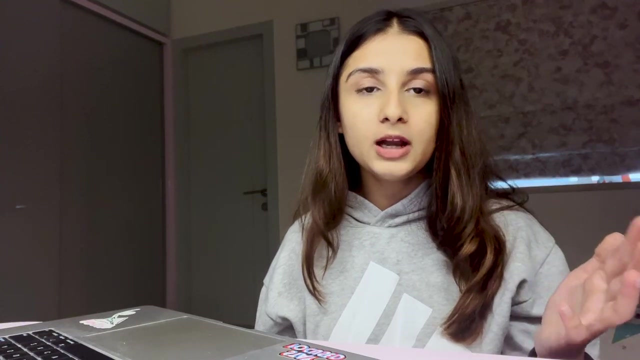 you'll be able to see how common bugs are fixed. so, in conclusion, i would like to say that, according to me, i think dvwa was the best resource for me to learn hands-on code reviews, and that was pretty much me doing it on my own. there was no blog that i was reading or following, apart from cryptocats. 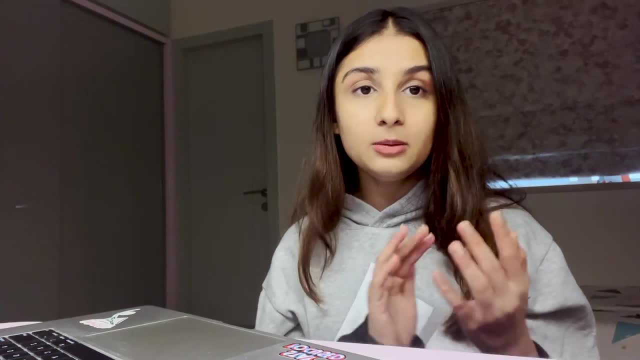 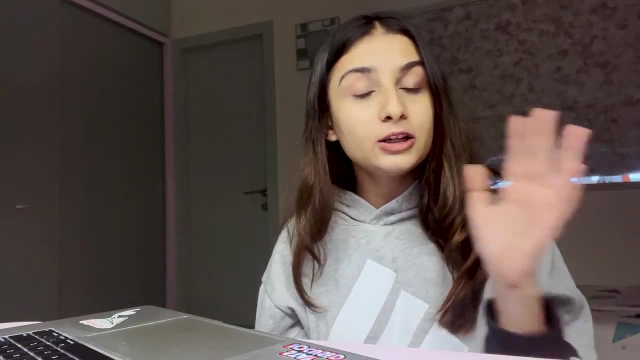 uh, youtube playlist. there was no other guide, so i think the best way to learn is to actually do code reviews and find vulnerable apps that you want to test and find bugs in them and then go to applications ui and see how the bug appears on the ui. so that's it for this video. i just wanted to